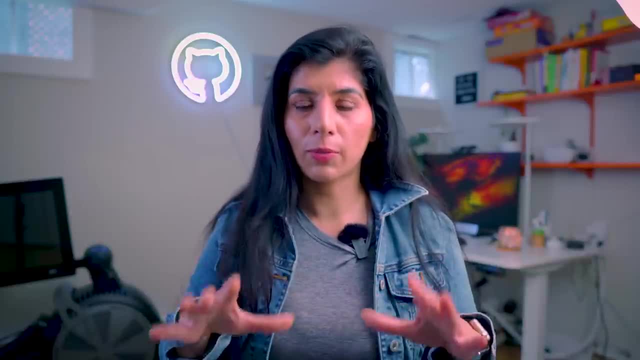 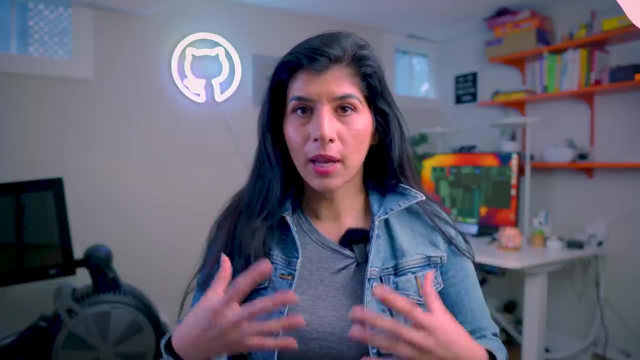 family has a place of its own. This video is just for the purposes of comparing the two job families and three things that I've specifically noticed. that makes data analyst job family stand out. Back in 2008, Harvard Business Review published this article where they call data scientists the 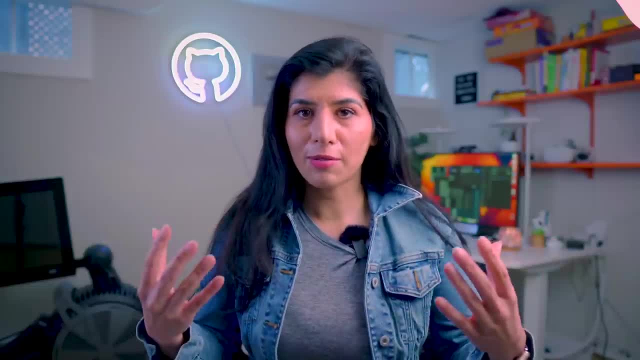 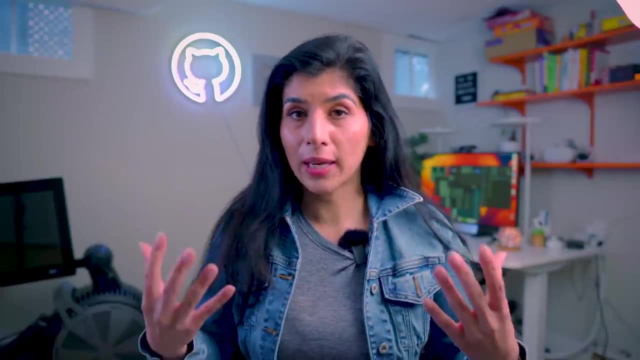 sexiest job of 21st century. Since then, data scientist job family has taken off and it is currently one of the most popular role out there. However, the job family is not perfect. You can talk to any data scientist who's working in the industry and they will tell you some of the big 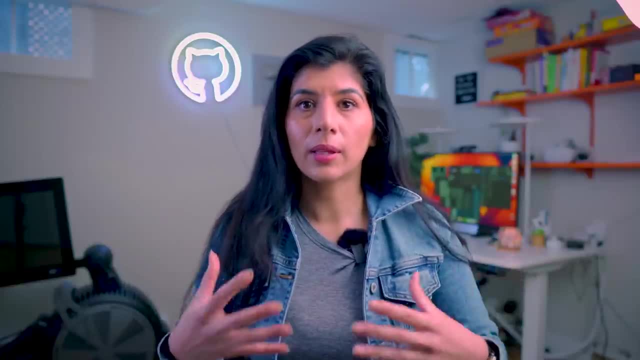 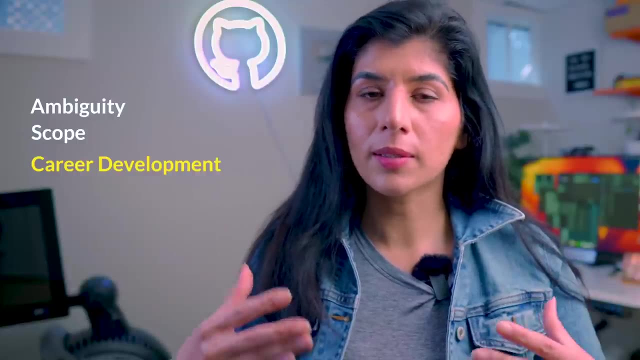 issues with the data science job family in the industry, starting with the lack of standardization, which leads to a lot of ambiguity, a very huge scope and makes it difficult to make progress within the career ladder and as well as make it difficult for job search purposes. So, before we, 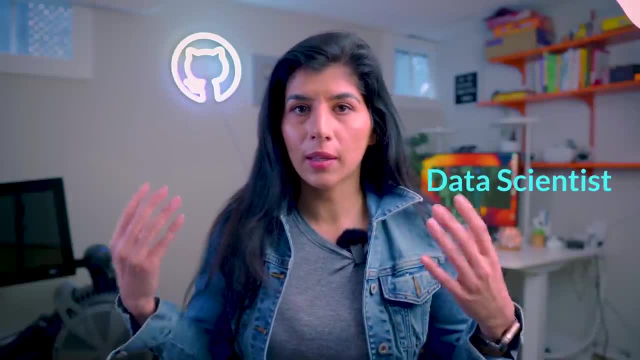 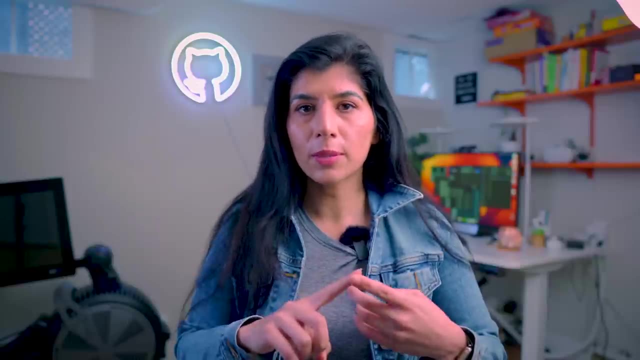 talk about the three reasons. I wanted to take some time to define the data scientist and the data analyst job family. to show you like what is different and what is similar. I'm going to segment the roles into four buckets and then I'll talk through each. The first bucket is math and 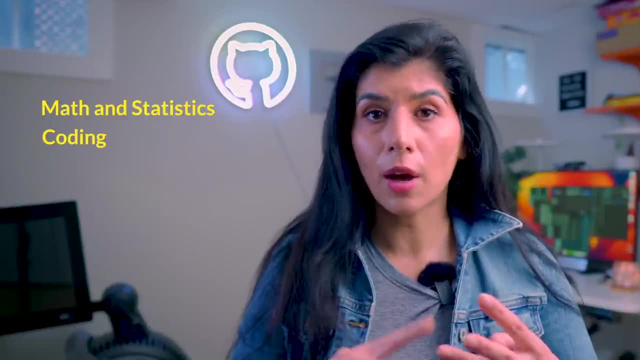 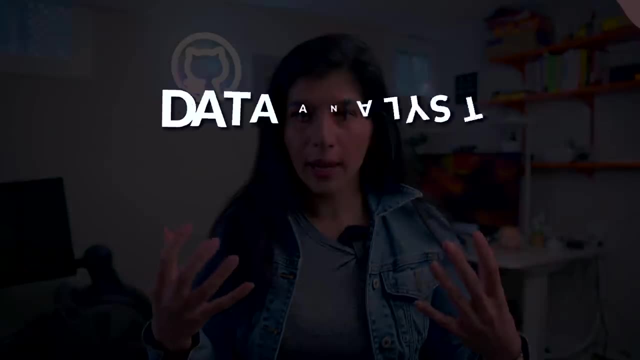 statistics. The second bucket is coding, The third bucket is software and tooling And the last one is my other bucket. So, quickly going through both of these job families, let's talk about math and stats. For a data analyst, you're expected to understand descriptive statistics. 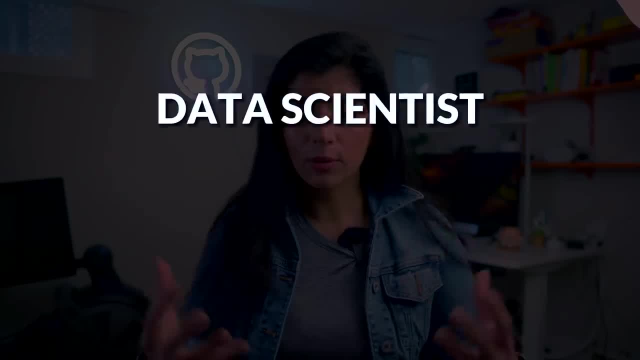 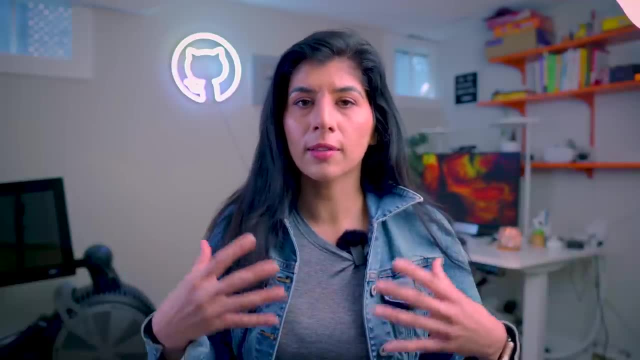 basic statistics and foundational math. For a data scientist role, you're expected to know advanced statistics, linear algebra, calculus and more. From coding standpoint, a data analyst is expected to know SQL- a bit of Python to complement your work in SQL, but in majority. 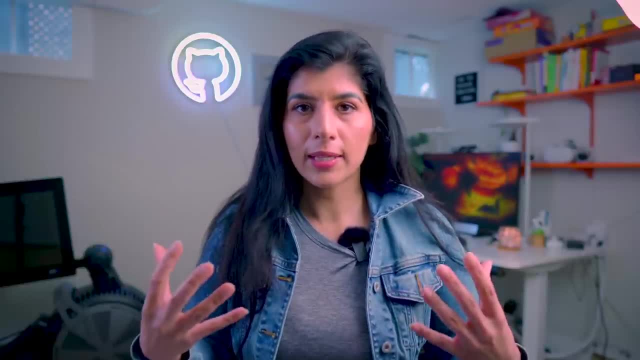 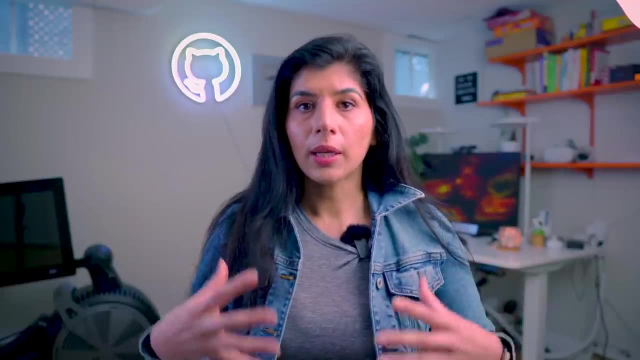 of the roles, data analysts primarily work with SQL. For data scientists, you're expected to know SQL, as well as scripting languages such as Python and R. In respect to software and tooling, data analyst is expected to know tools such as Excel. 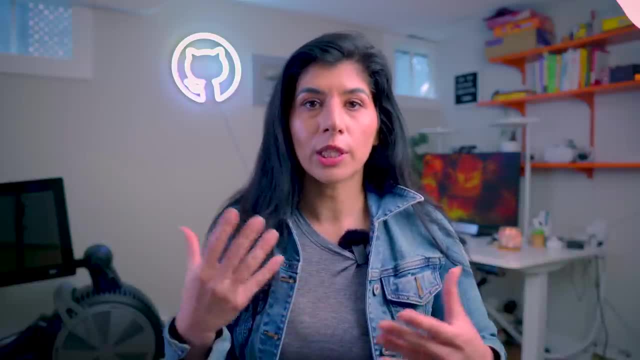 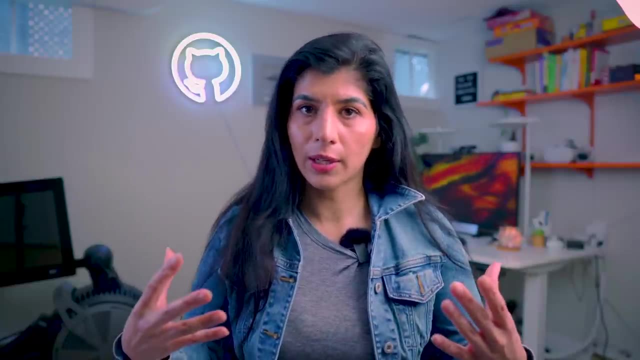 Google Sheets. For visualization, they're expected to know tools such as Tableau, MicroStrategy, Power BI and ETL. For data scientists, you're expected to know ETL, on how to extract your data, where the data lives, And for the tools, you're expected to know RStudio, if 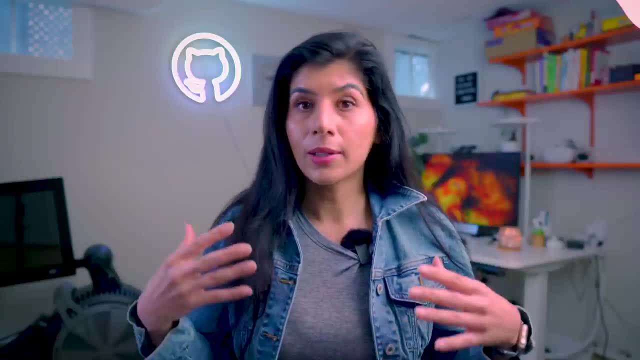 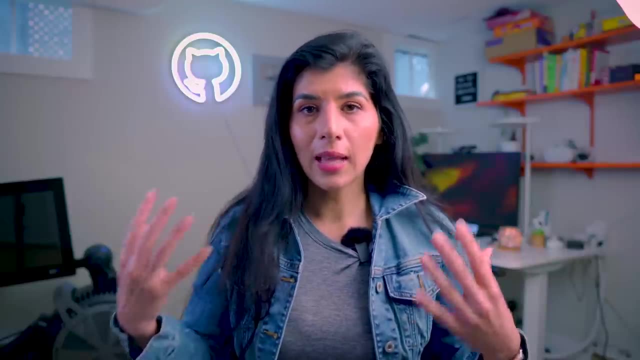 you work with R Jupyter Notebook, Google Colab Notebooks, understand how to work with code reviews, understand how code review process works and to be able to do it on your own. And the last in my other bucket for data analysts: you're expected to have good communication and 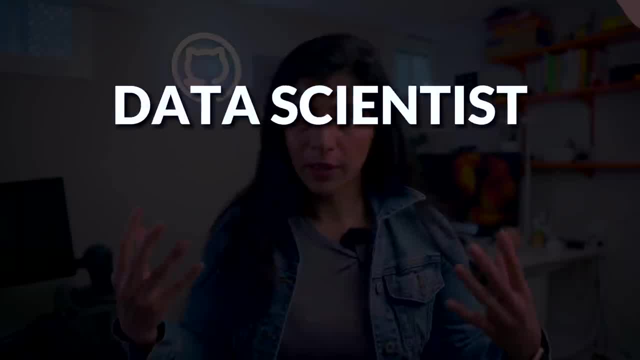 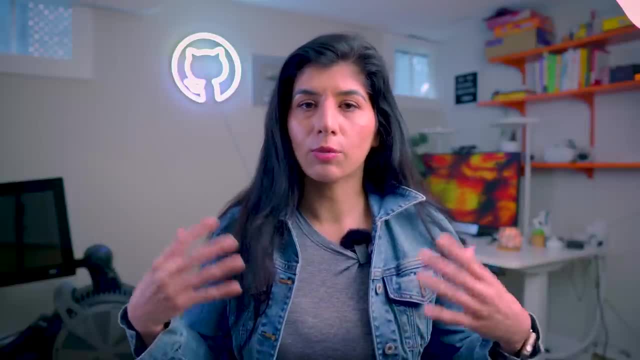 analytical skills, problem solving skills. For data scientists, you're expected to have good communication skills, problem solving skills and having a good business understanding. So in my other bucket, basically the required skills for data analysts and data scientists is both: Now that we understand like, what are the core skills required for both roles? 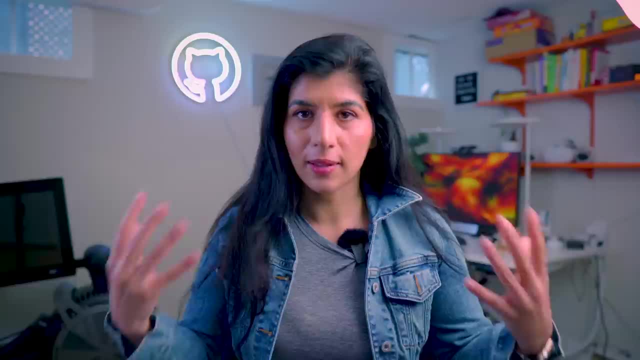 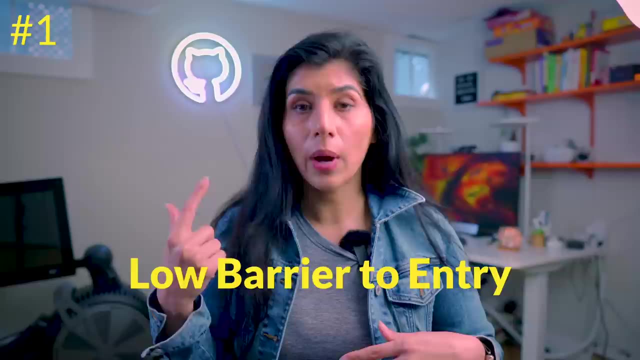 let's talk about what makes data analyst job family better than data scientists. There are three reasons. primarily, data analysts might be a better fit for you. Number one is that the job family has low barrier to entry For a data scientist role. most cases you're expected. 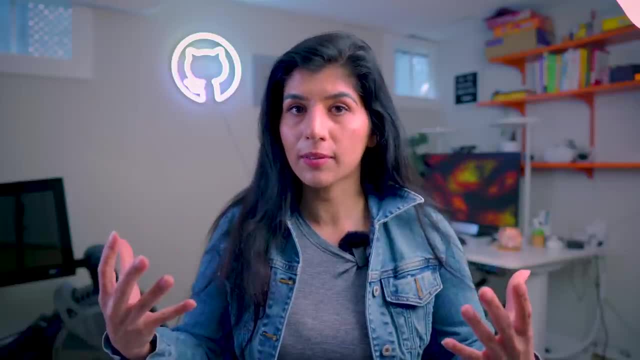 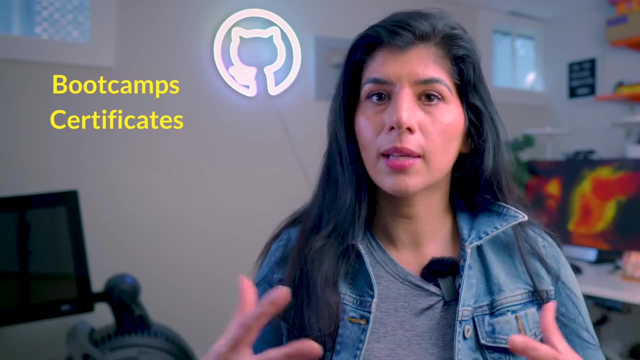 to have a master's degree or PhD in a lot of cases, Whereas for a data analyst role, PhD is not one of the requirements. There are a lot of data analysts who have taken bootcamps, certificates, online courses, as well as bachelor and master's degree to enter the field. There is 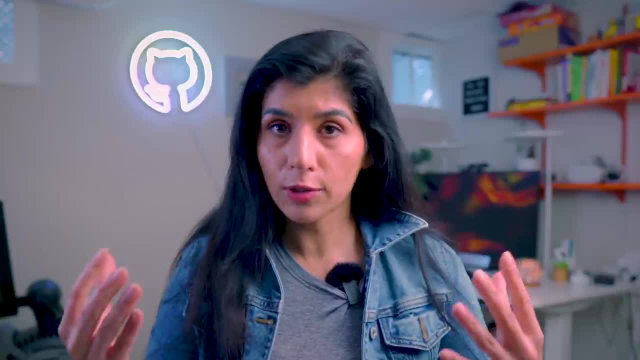 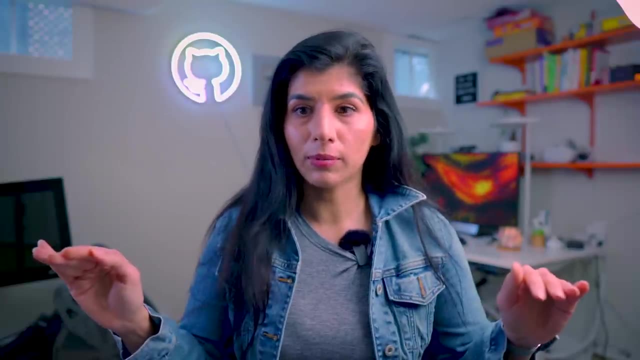 a wide variety of entry points for a data analyst role. Now, that also means that if it's low barrier to entry, that means a lot more people will enter and then there will be a lot of competition. But that's not the point of this conversation. Yes, that might happen, But at the same time, 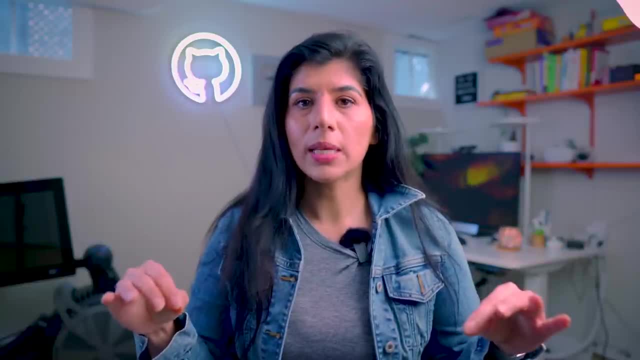 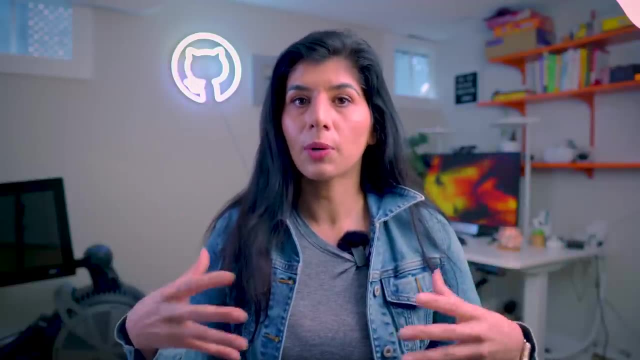 your barrier to entry is lower than a data scientist role, which means that it would be for somebody who just wants to get into data analytics. it would probably be if you're planning to do a self teaching route. Data analytics is something that you might be able to teach on your 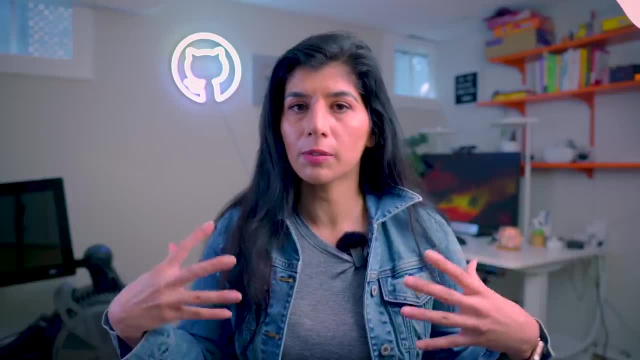 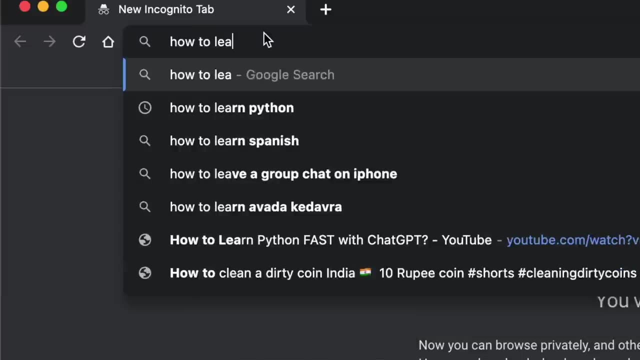 own or take certain online certificates and courses to help yourself prepare for the role. Talking about data analyst and data scientist toolkit, one of the common skills that both roles need to learn is Python, And I found this free ebook to learn Python that I wanted to share. 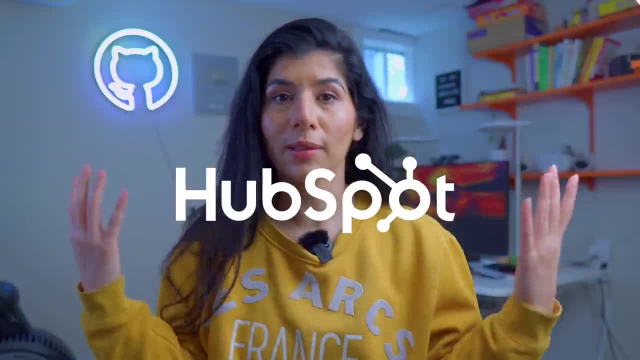 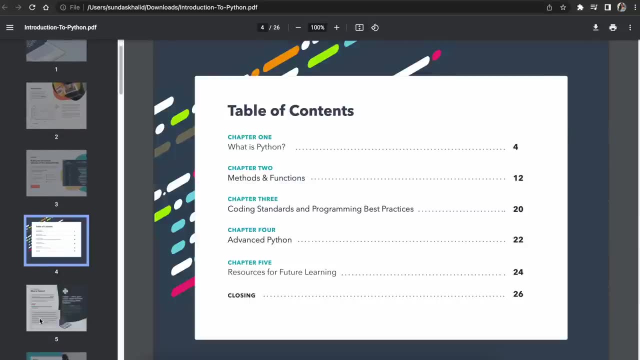 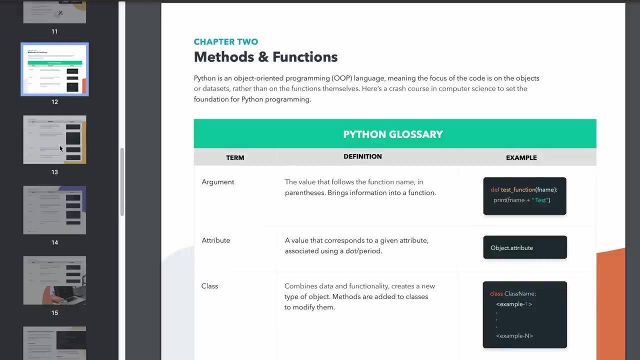 with you all. The ebook is created by HubSpot, who is sponsoring this section of the video. In this ebook, you'll find introduction to Python with the lens of data analytics and get educated on libraries such as pandas, numpy and more. What I really like about this ebook is that it breaks down Python concepts in very simple. 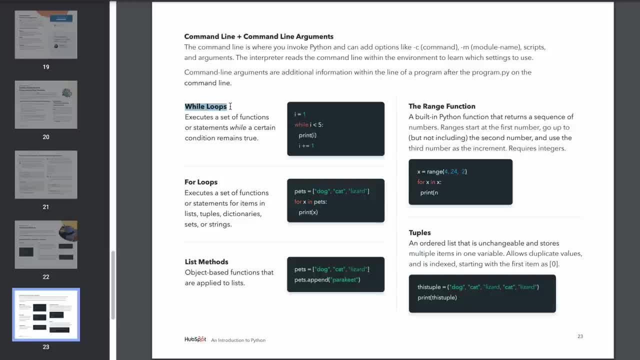 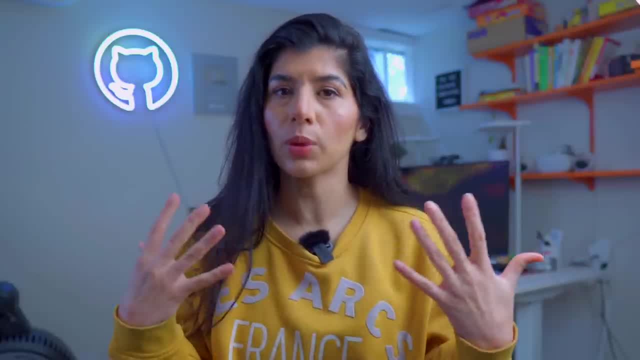 fashion. For example, while loop is one of the concepts in Python that is not very intuitive to get at first, But if you read the examples given in this ebook, it goes into a lot more detail. I'm linking the ebook in the description below. It's available to download for free, thanks to HubSpot. 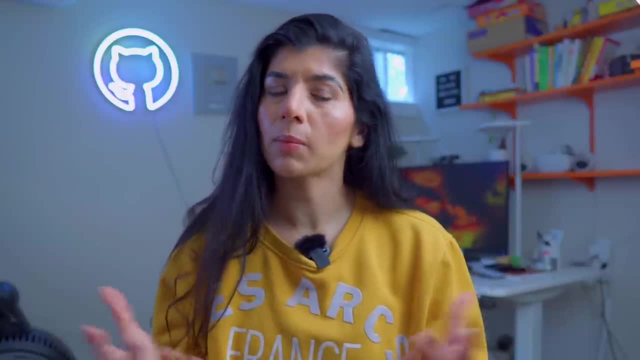 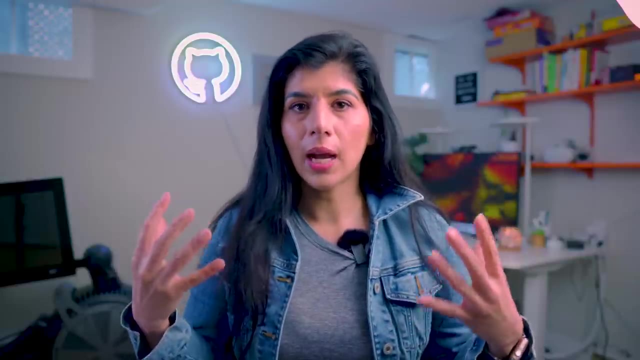 And now let's talk about the reason number two why data analytics might be a better career choice for you. The second reason why data analytics might be a better fit for you is in data analytics, oftentimes you are building tangible things. For example, you are building dashboards. 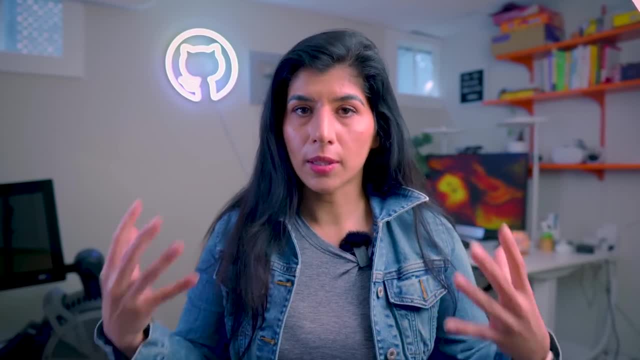 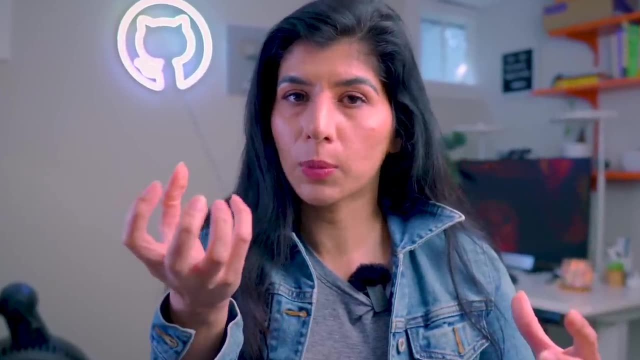 you're building reporting. In a data scientist role, you're often doing advanced statistics and building models and using machine learning. A lot of your work tends to be research focused. Many times there is no tangible output that can point to show your impact, Whereas in a data analyst role you actually have. let's say, 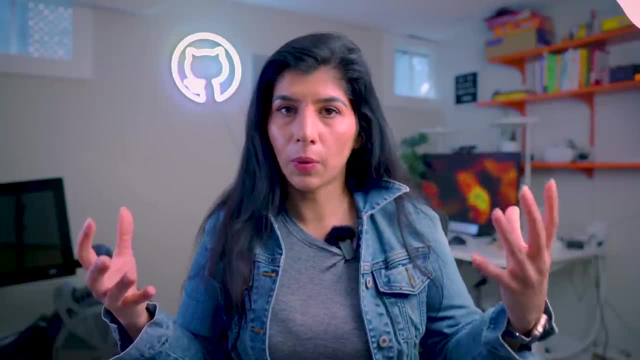 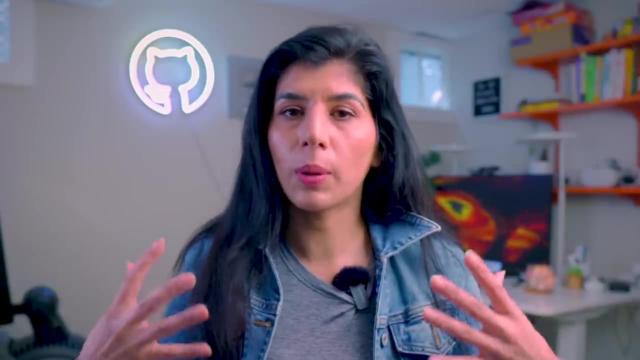 if your work requires you to build dashboards or your build report, you're able to have tangible artifacts that you can show to prove the value of your work, And if you're the type of person who enjoy building tangible things, then data analytics might be a better fit for you than. 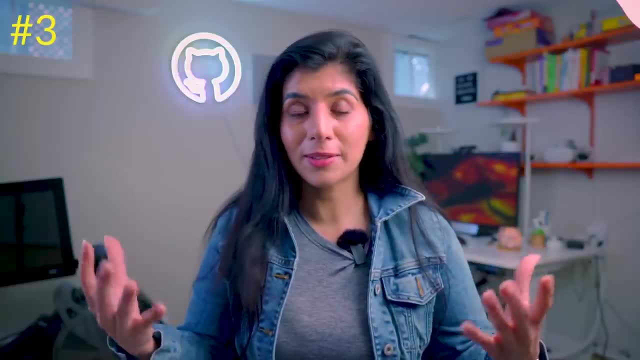 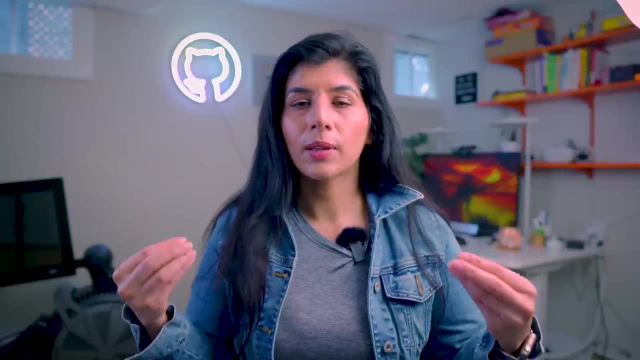 a data scientist role. The third, which is one of my favorite reasons to consider data analytics role, is the scope and the standardization of the job family. For a data scientist role, the job family is not standardized. Oftentimes a data scientist at company A does. 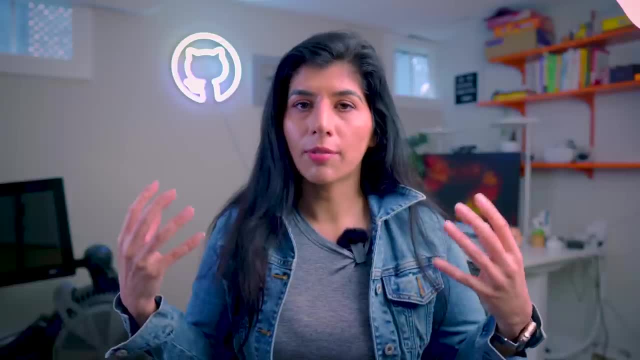 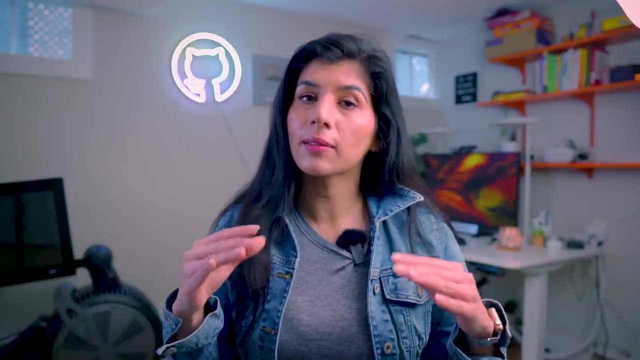 not translate well to a data scientist at company B, which leads to a lot of ambiguity and it makes it difficult to job search as well. For a data analyst role, however, things are way. it's not perfect, but it is more well-defined than a data scientist role, In that case, a data analyst at 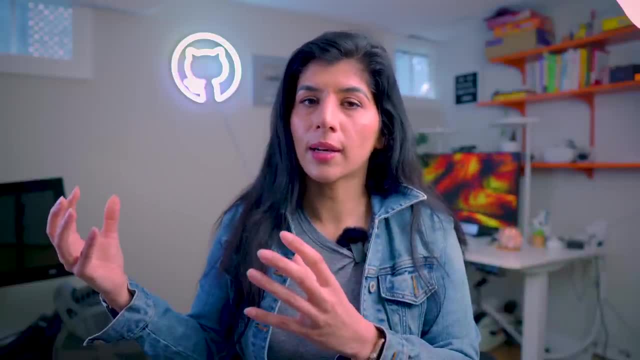 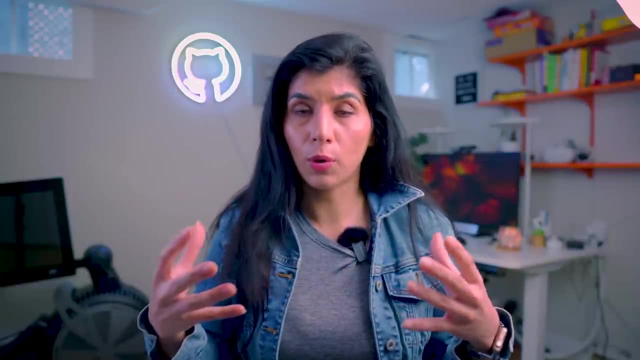 company A is going to easily translate to a data analyst at company B, which makes your interview process easier And within the company, you are also able to have a better understanding of your scope and able to work toward making a progress in your career. I do hope that the data 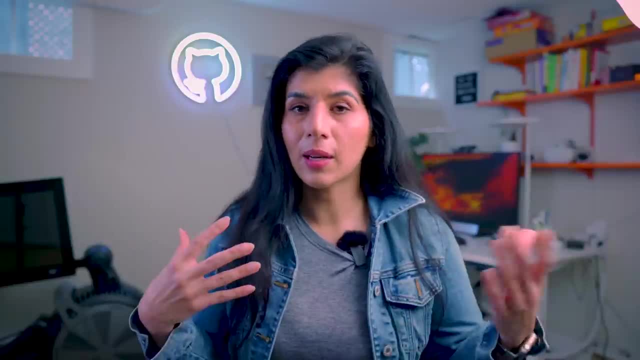 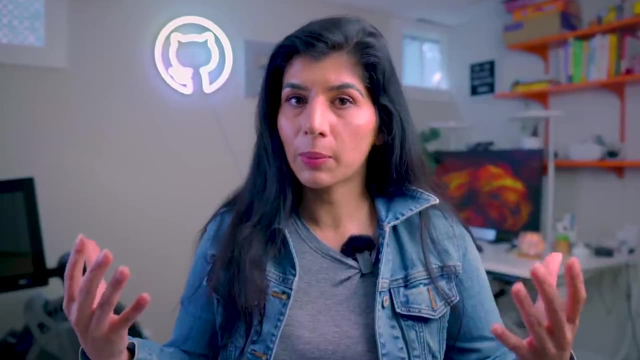 scientist, job, family eventually comes to a point where data scientist at company A and B means the same thing. but we're not there yet. So I know these three points might not be that big of a deal for everybody, but it might be a big deal for somebody Again. the last point that goes without.